And each state has its own unique natural attractions that cater to different outdoor enthusiasts. Now, when it comes to history, both states played significant roles in the early colonization of the United States of America. North Carolina was home to the famous Lost Colony on Roanoke Island and was one of the original 13 colonies Now South Carolina. 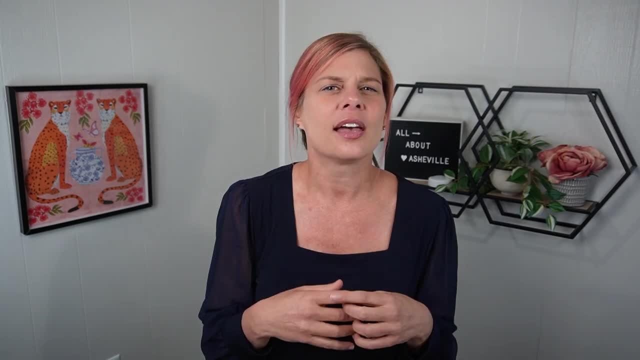 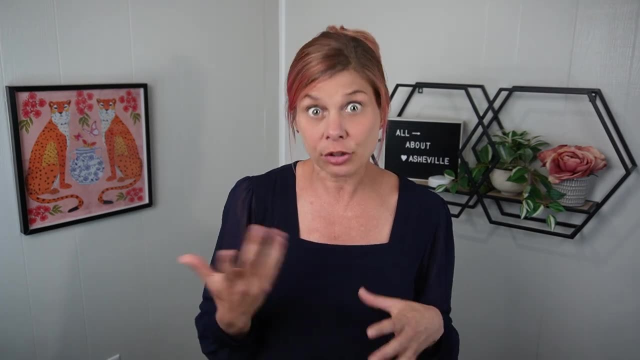 on the other hand, was one of the first English colonies in the region and played a pivotal role in the American Revolution. The state also has a rich African-American history, particularly in Charleston, where it was a major port during the slave trade North. 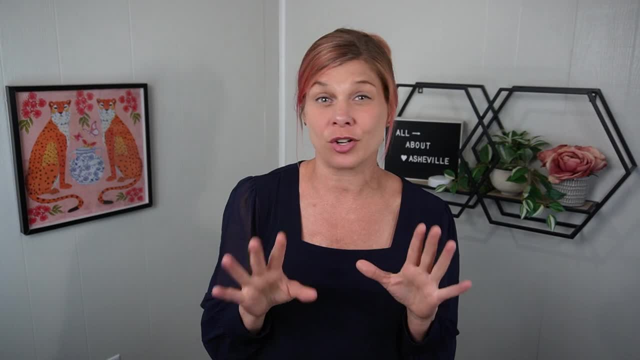 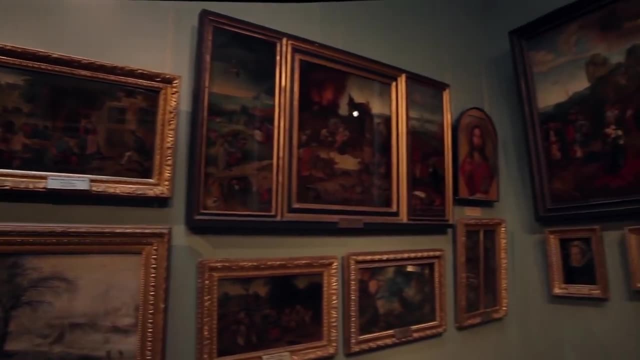 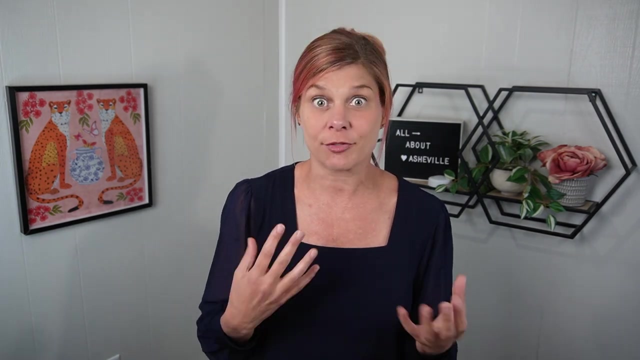 Carolina and South Carolina both boast unique and vibrant cultures. North Carolina has a diverse art scene with famous pottery tradition in Seagrove and the Biltmore Estate in Asheville and a strong bluegrass in Folkmuse music, heritage stemming from the Appalachian region. 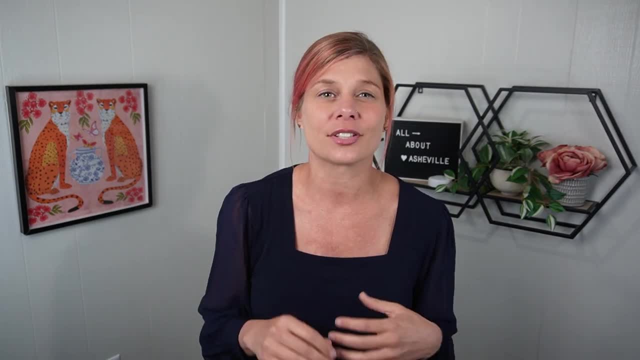 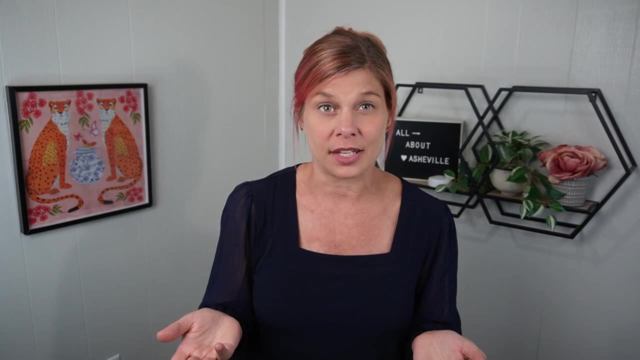 South Carolina, known for its southern charm, offers a rich Gullah Geechee culture in the Lowcountry region. Then they are celebrated in annual events like the Spoleto Festival in Charleston and the delectable cuisine like shrimp and grits. Mm, a personal favorite. Each state showcases its own distinct cultural flavor. The Native American heritage on both the North Carolina and South Carolina side is a vital part of the state's cultural fabric. The indigenous people who originally inhabited these lands have a rich and diverse heritage. 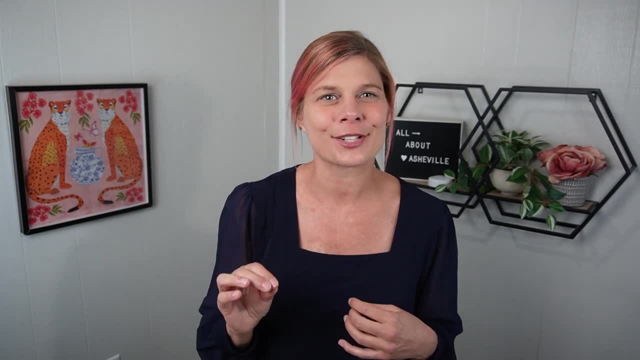 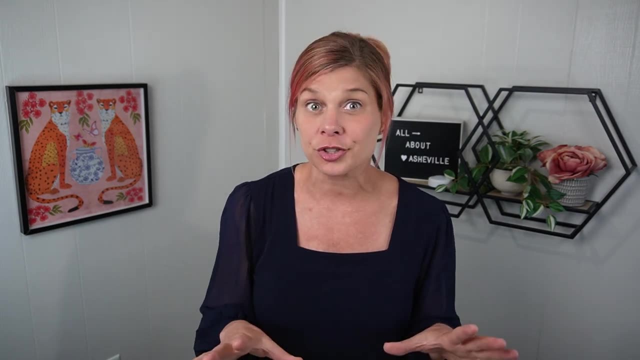 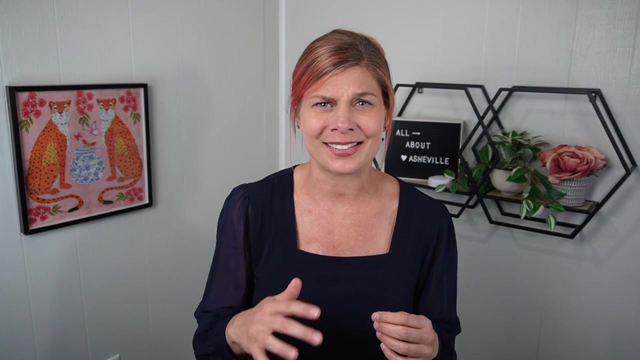 that continues to influence the region. Now let's explore some of the notable cities in both North Carolina and South Carolina. These states are home to vibrant urban cultures that have historical landmarks and a range of amenities. North Carolina boasts several dynamic cities that showcase a blend of modern and southern charm. 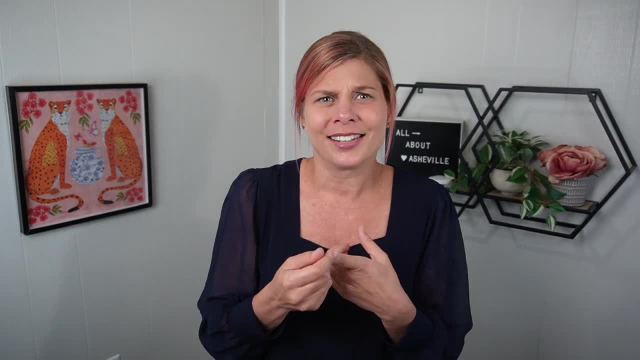 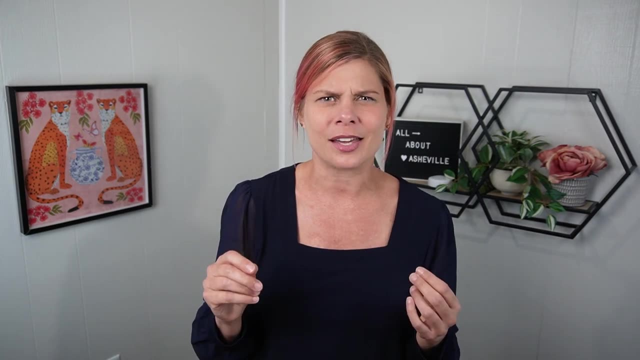 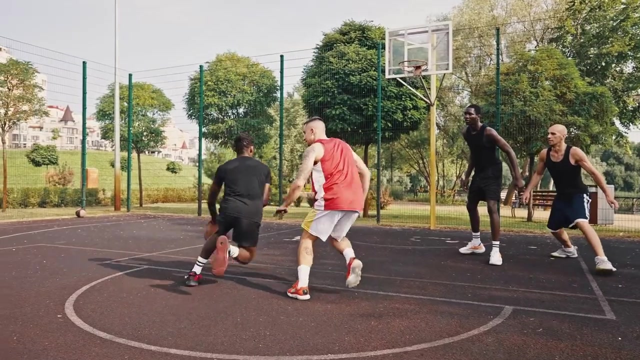 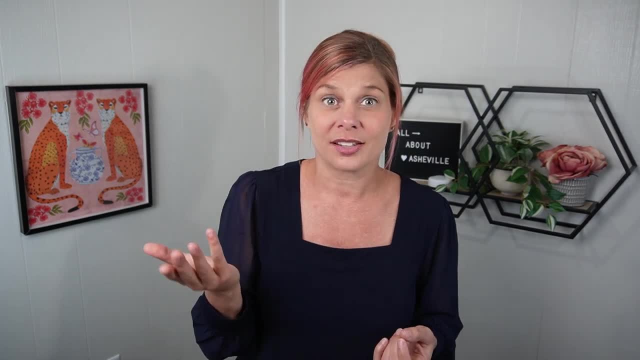 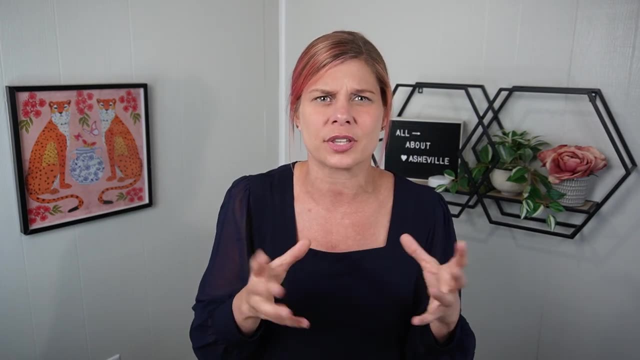 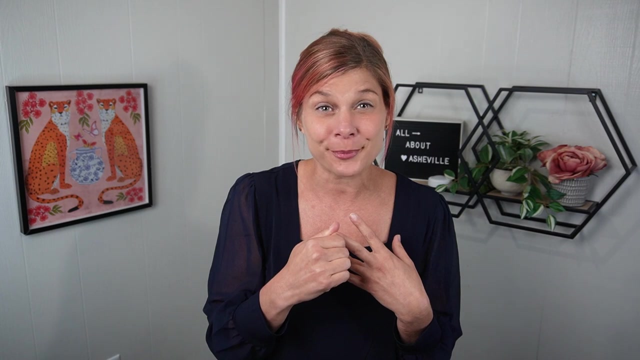 And it's known for its research institutions, like the North Carolina State University, And it has a really strong mix of historical sites, such as the North Carolina State Capitol, contemporary art galleries, a lively downtown known as Fayetteville Street, And then there's Asheville, my personal favorite. 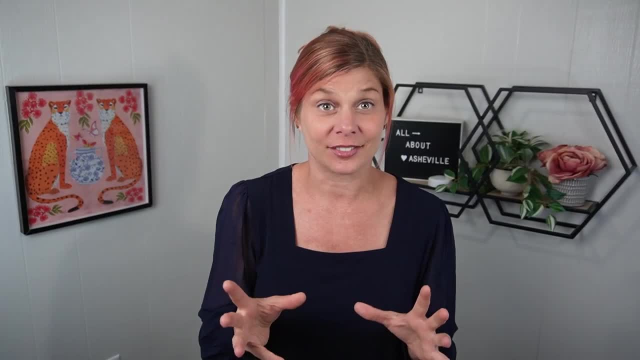 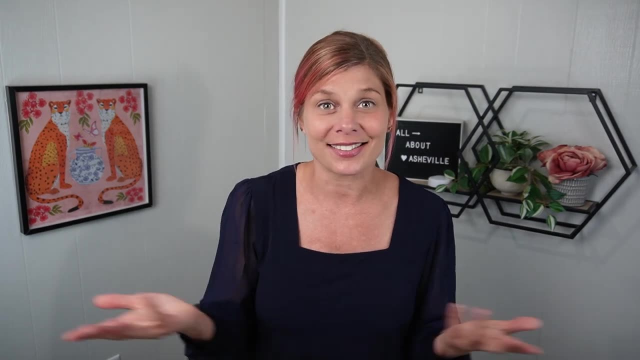 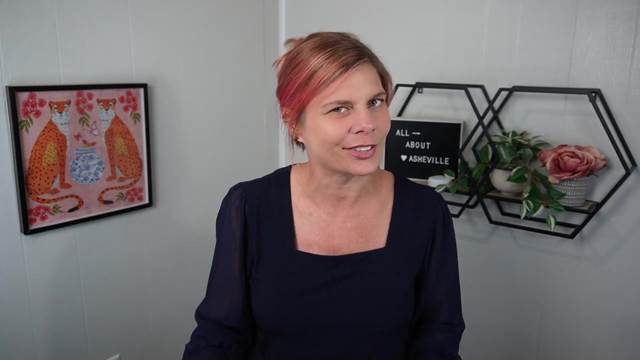 Nestled in the Blue Ridge Mountains, Asheville is a vibrant city Renowned for its artistic and bohemian atmosphere and known for its eclectic downtown and the Biltmore Estate and access to outdoor activities like hiking and the Appalachian Trail. And it is just definitely my personal favorite. Wink wink. South Carolina is home to cities that exude Southern hospitality and they showcase rich historical heritage. And they hear some of the notable cities in South Carolina, like Charleston, known for its well-preserved historic district and cobblestone streets. 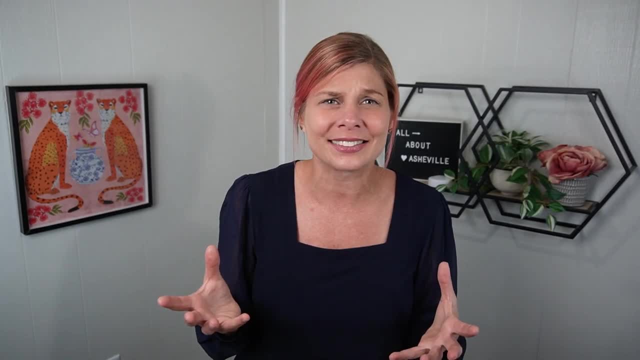 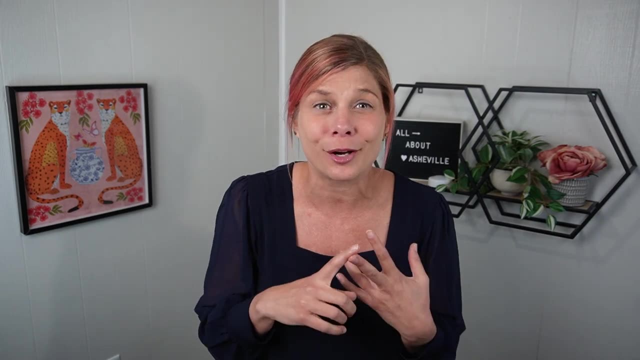 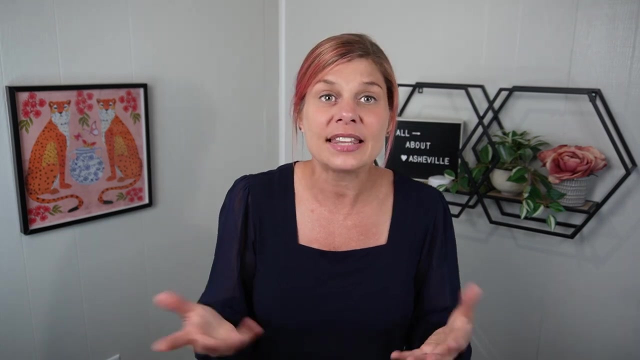 Charleston is a city that's steeped in charm and elegance, And it has such interesting architecture and iconic landmarks like the Battery and Rainbow Row. The city offers a vibrant food scene and beautiful nearby beaches, even with surf in some areas. And then there's Columbia. 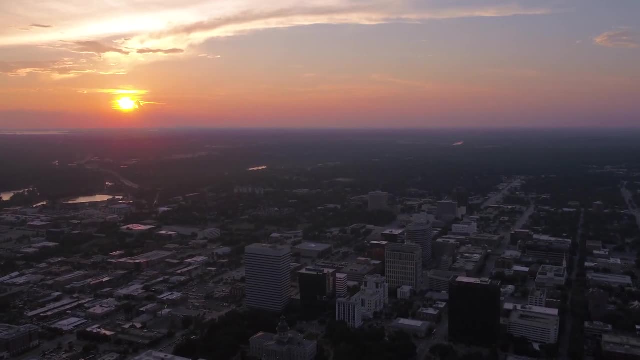 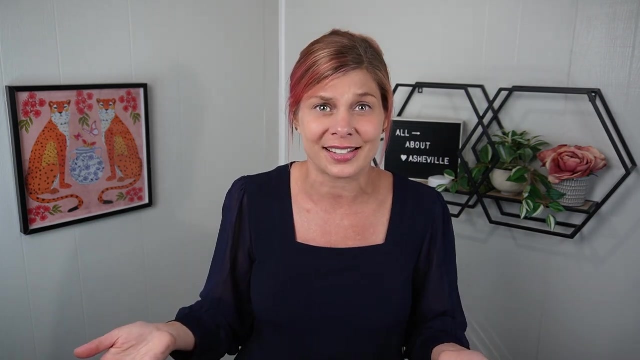 serving as the capital of South Carolina, And Columbia is a city with a diverse blend of history as well and culture and outdoor activities. It's home to the University of South Carolina and features attractions like the State House and the Riverbank Zoo and the Garden and the Columbia Museum. of Art. And then there's Greenville, South Carolina, located in the foothills of the Blue Ridge Mountains, not too far away from Asheville, And Greenville has really transformed into a vibrant and progressive city. It offers a revitalized downtown and a thriving art scene. And it has a range of outdoor recreational opportunities as well. Now, when it comes to the cost of living, both North Carolina and South Carolina offer affordability compared to other states. However, South Carolina tends to have a slight edge in terms of the cost of living. 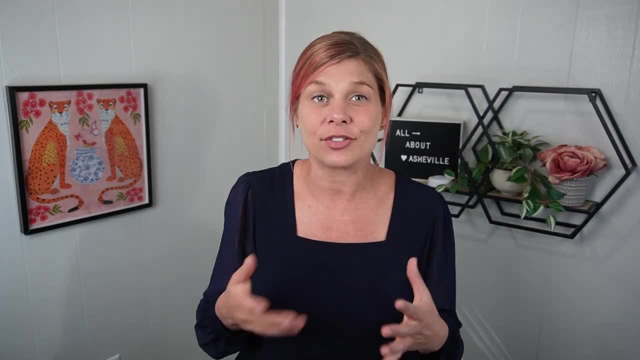 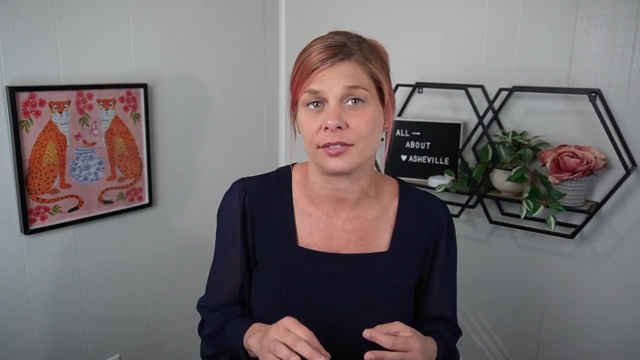 And that's because of overall affordability. Housing taxes and everyday expenses are often a little bit more budget-friendly in South Carolina, making it an attractive choice for those seeking a lower cost of living. Both states have reputable education institutions, But North Carolina stands out with its renowned universities. 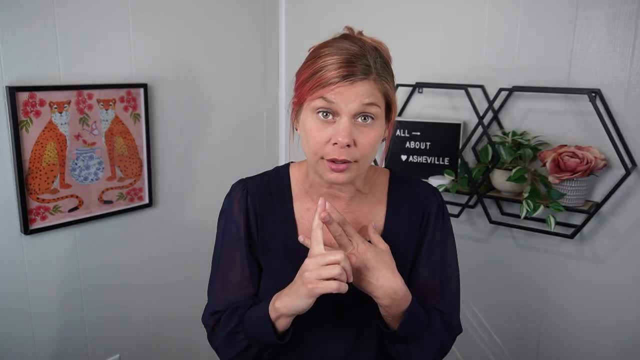 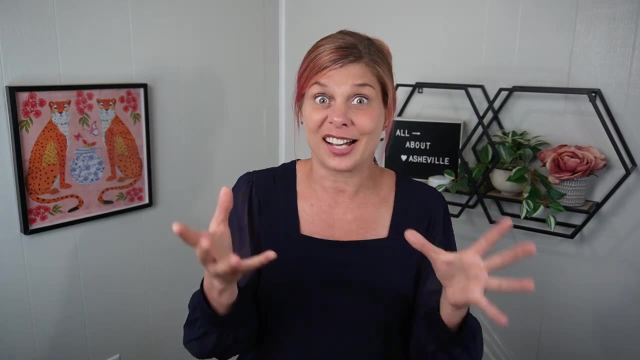 like Duke University and the University of North Carolina at Chapel Hill and North Carolina State University. Those are just a few of the prestigious academic institutions that are housed in North Carolina. While South Carolina has a very strong education system, North Carolina also has notable universities. 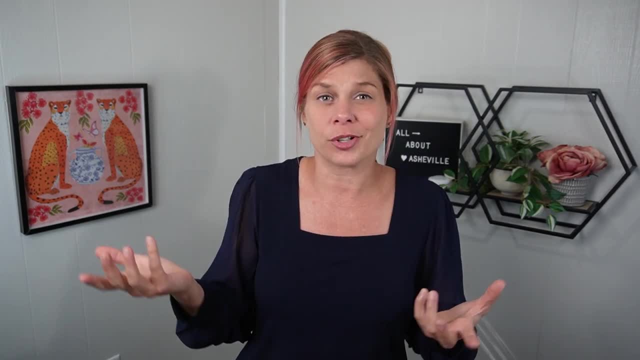 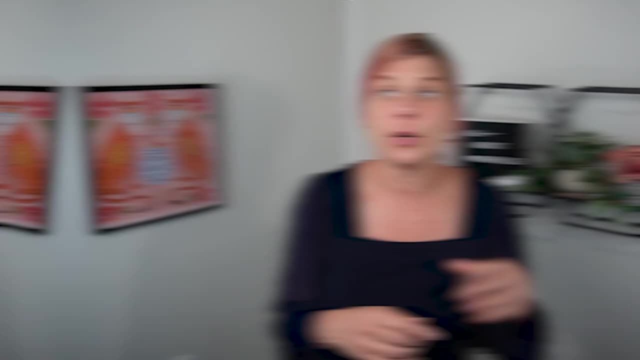 such as Clemson and the University of South Carolina, And North Carolina has a broader range of higher education options and is often considered a strong contender in this category. Both North Carolina and South Carolina offer appealing destinations for tourists. North Carolina is known for its beautiful 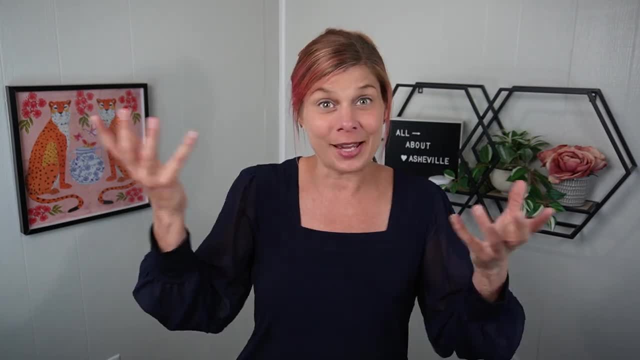 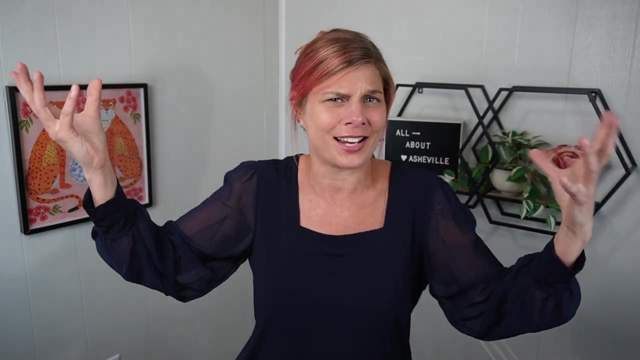 breathtaking views and landscape and the Outer Banks And the state again attracts like outdoor enthusiasts, people who want to spend time in nature, And beach goers and hikers. And South Carolina, on the other hand, has also a stunning coastline and historic cities. and popular tourist attractions in itself, like Myrtle Beach. Each state has its unique charm and caters to different interests and preferences, And if you're into sports and they play a significant role in your life, the culture in both North Carolina and South Carolina could be of. 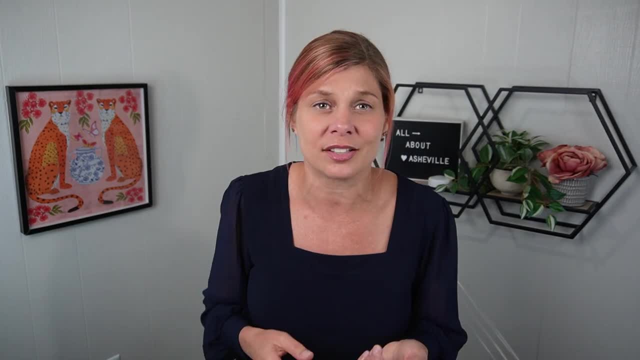 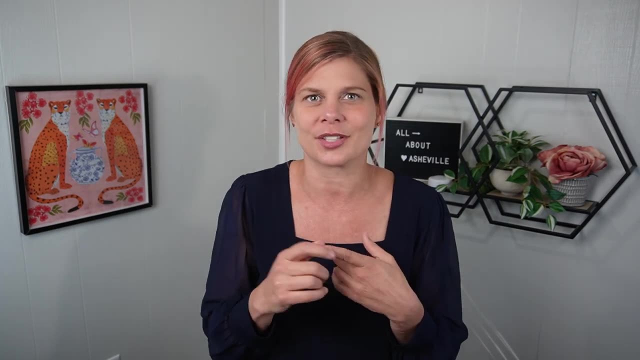 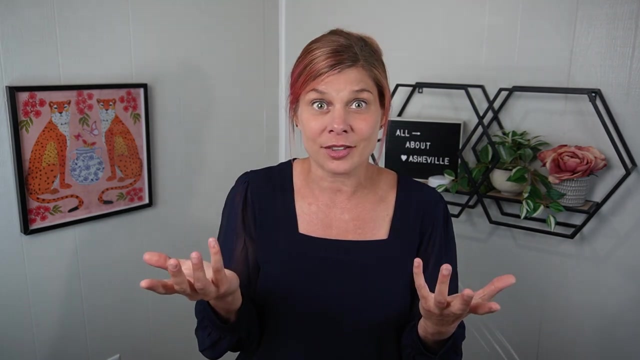 interest. So you probably already know this, but North Carolina is famous for its passionate fan base of college basketball teams like the Duke Blue Devils and the University of North Carolina Tar Heels, And the state also has a professional sports team, including the Carolina Panthers and the NBA's Charlotte Hornets. South Carolina, on the other hand, while not home to major professional sports teams, has a strong following, particularly for the University of South Carolina Gamecocks. You don't want to get in their way. Sports are a unifying force in both states. 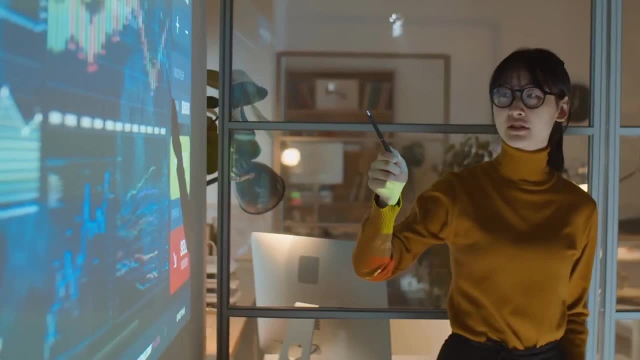 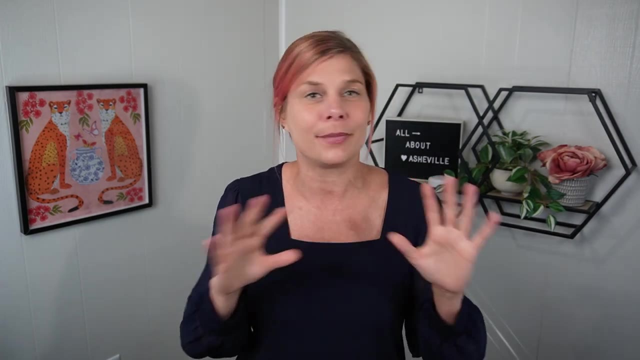 and they can bridge communities together. Now, when we're thinking about economic opportunities, North Carolina has the upper hand. It has vibrant cities like Charlotte and Raleigh, which serve as major economic hubs. The state offers a range of industries, including technology and finance. and research. South Carolina, while making major strides in the economic center, has fewer major urban centers and a more limited job market compared to North Carolina. However, South Carolina has a strong manufacturing presence, particularly in aerospace and automotive industries. The Carolinas are really blessed when it comes to natural landscapes, and they beckon that adventure. 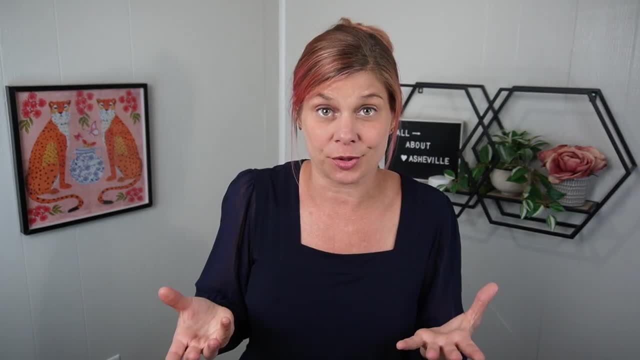 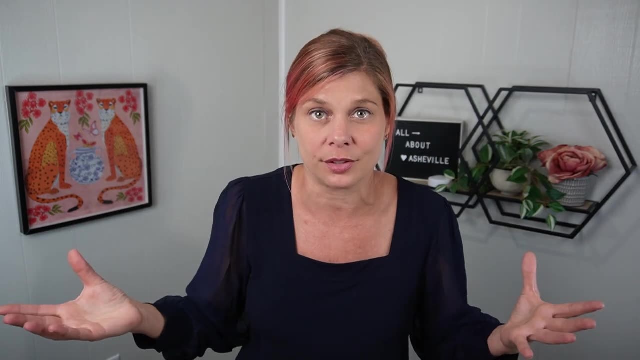 inside of us, And you can't forget the Blue Ridge Parkway that goes right through there, which is a scenic drive that goes for miles and miles through mountains and offers breathtaking viennent vistas and views. Motorola offers a superiorК And there's such state parks like Hanging and Rock and Pilot Mountain. South Carolina also has national parks and nature conservation. You not only have a place to stay in your home state, but the state also offers great opportunities to live there, be located in the faunt of your home state. 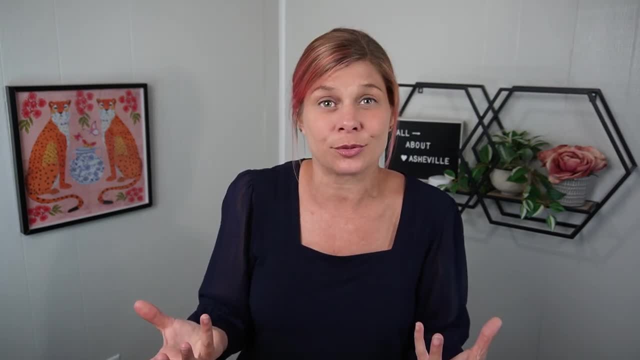 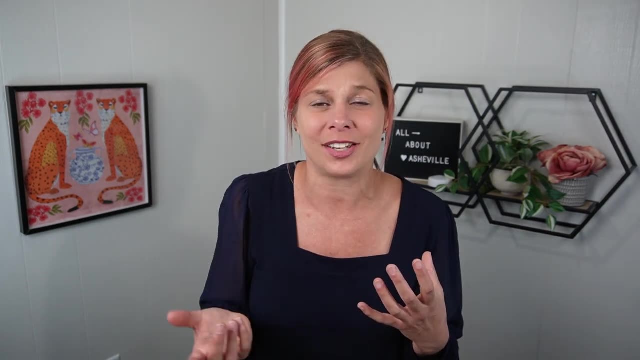 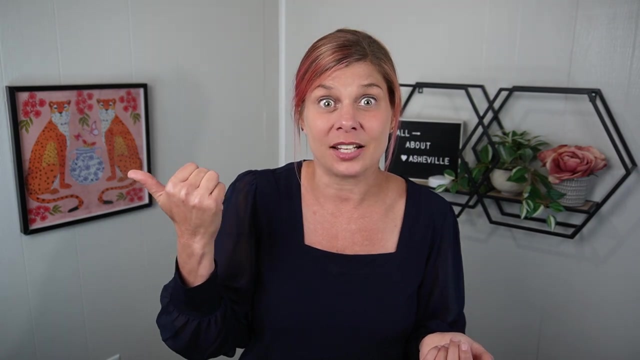 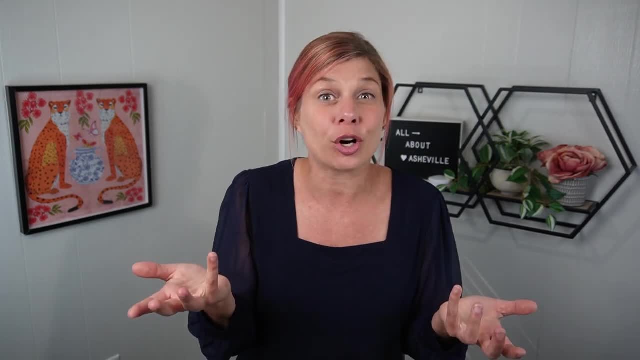 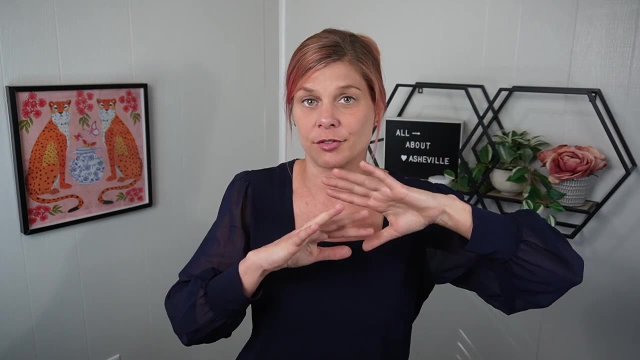 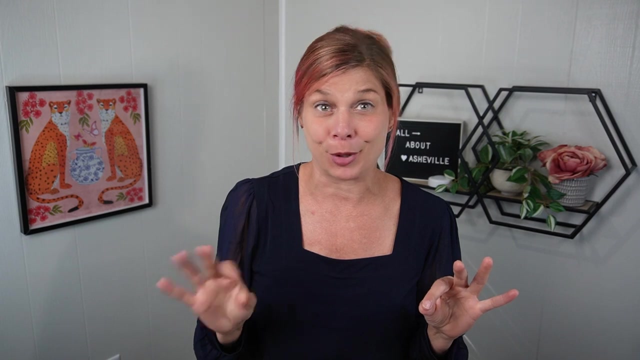 and lakeside dining. and then the one that I'm really familiar with is Lake Hartwell between. it's on the border between South Carolina and Georgia, and it's a massive reservoir covering over 56,000 acres, and there's boating and water sports. now let's dive into the coastal delights of both states. they 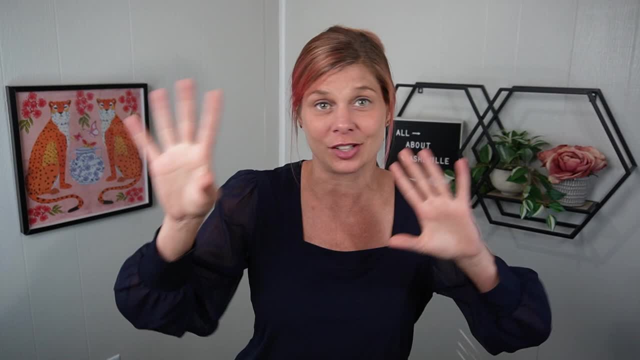 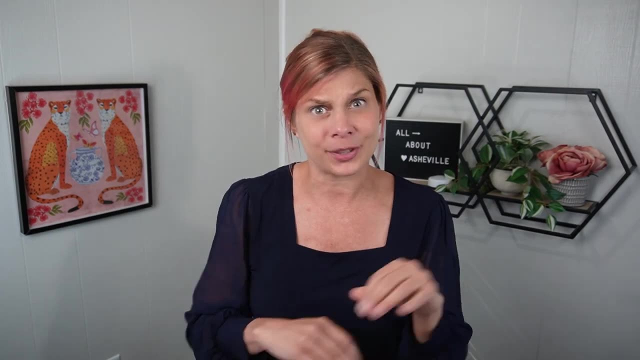 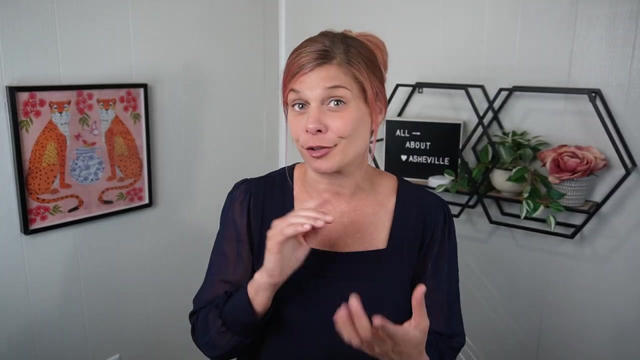 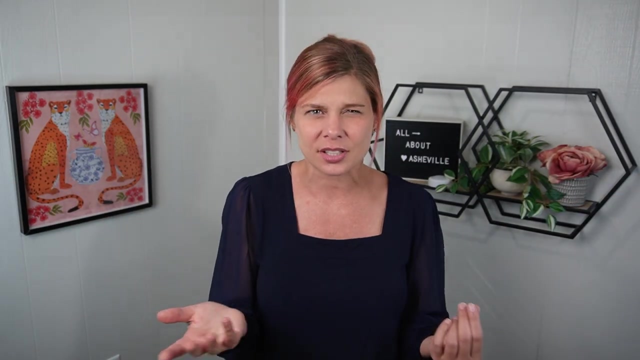 both have beautiful beaches, offering opportunities along the Atlantic Ocean for sand and sun and fun and recreational activities. now North Carolina is blessed with a stunning coastline and a variety of different beaches, and a few notable beaches in the area are the Outer Banks, which stretches over 200 miles. there's barrier islands and pristine beaches and lighthouses and a lot. 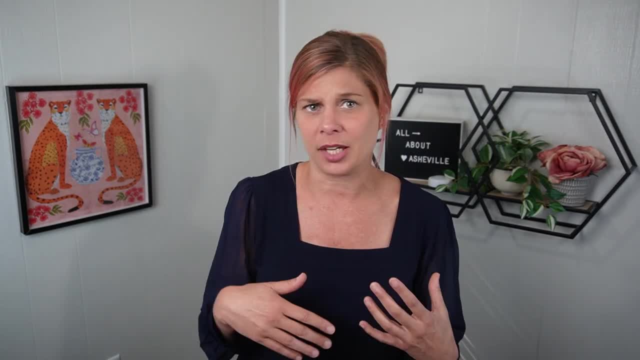 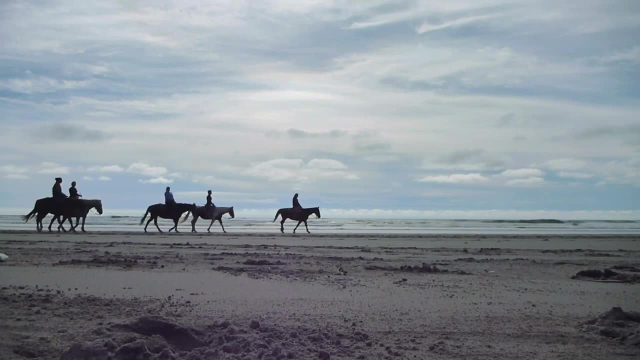 of rich history and it offers opportunity for swimming and kite boarding, and it also has wild horses that just run free on the beaches and it's absolutely gorgeous. it's like another world sometimes. it has a strong culture and a really strong community as well, and then there's 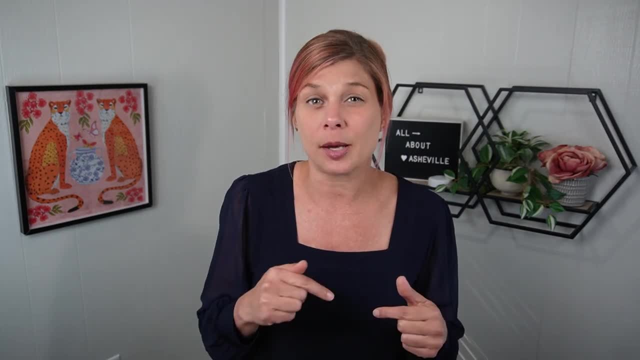 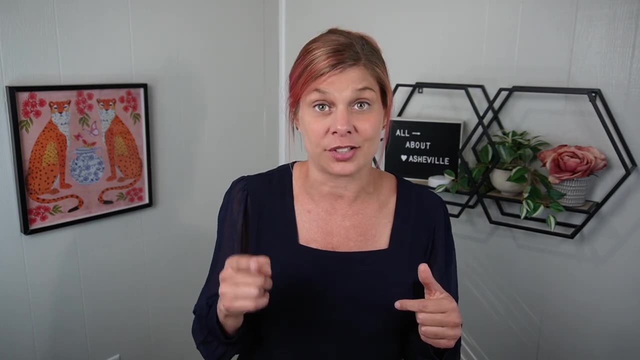 Wrightsville Beach, which is located near Wilmington, and this is really a popular destination for white sandy shores and crystal clear waters, and it has a vibrant beach scene um, with kite boarding and kayaking and paddle boarding, and a lively social atmosphere as well. they really know how to have a 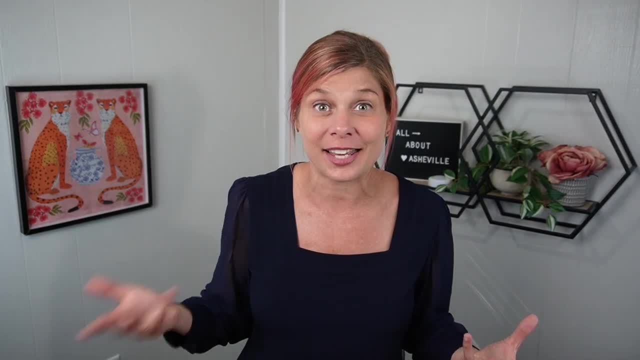 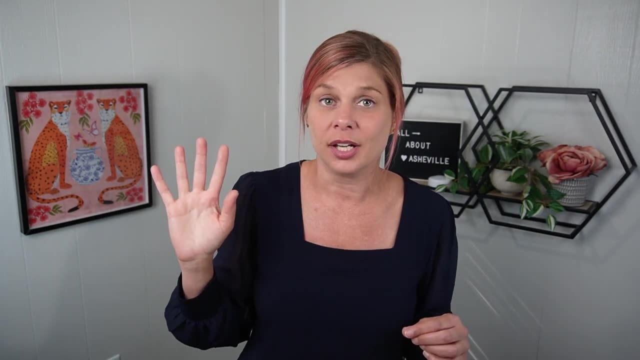 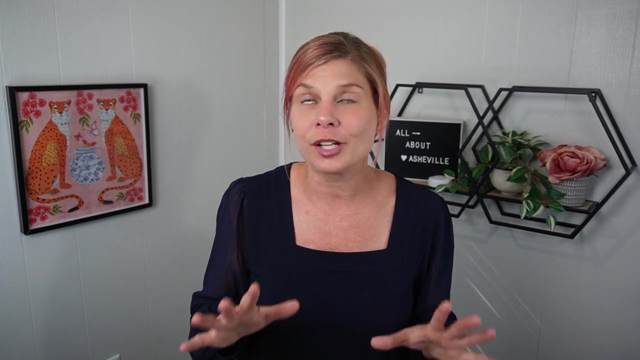 good time there. there's Cape Hatteras National Seashore as part of the Outer Banks. Cape Hatteras is the National Seashore, uh protected coastline that has just beautiful uh beach combing and bird watching opportunities and it's just really unspoiled. you feel like you are in the middle of nowhere. 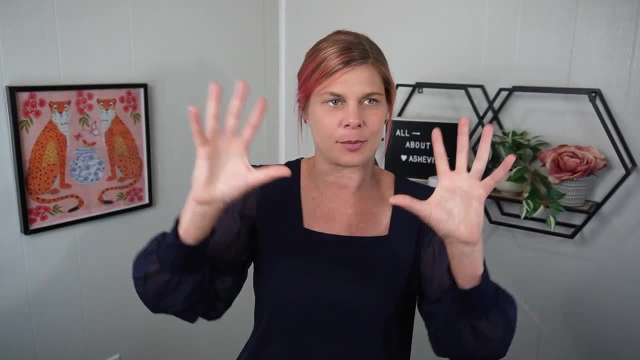 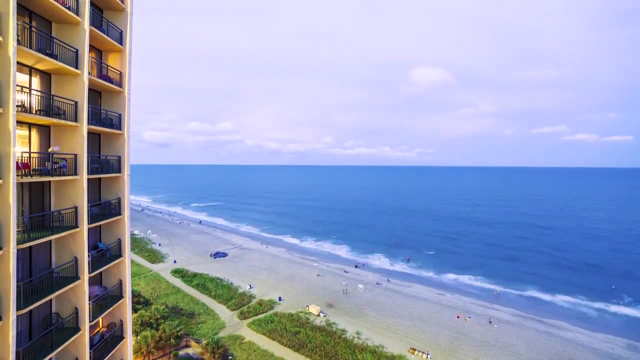 because there's these rolling sand dunes and it's just like you can take a picture. it looks like you're just floating in the sky now. South Carolina is equally blessed with picturesque beaches that cater to a range of interests. there's Myrtle Beach, which is a renowned vacation destination. and offers uh lively beachfront boardwalks and entertainment options like amusement parks and water parks and golf courses. and then there's Hilton Head Island, which is located right off the southern coast of South Carolina, and Hilton Head is a really popular beach destination Island and it has wonderful beaches and golf courses and resorts and there's kayaking and fishing and exploring all kinds of nature scenic trails. Kiowa Island is another one. it's a polluted and luxurious beach getaway, known for its natural beauty and upscale amenities, and marshlands teeming with wildlife and championship golf courses as well. South Carolina often wins in terms of affordability, while North Carolina really shines with higher education and economic. 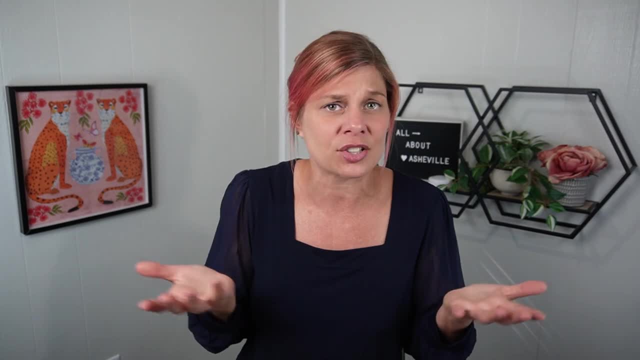 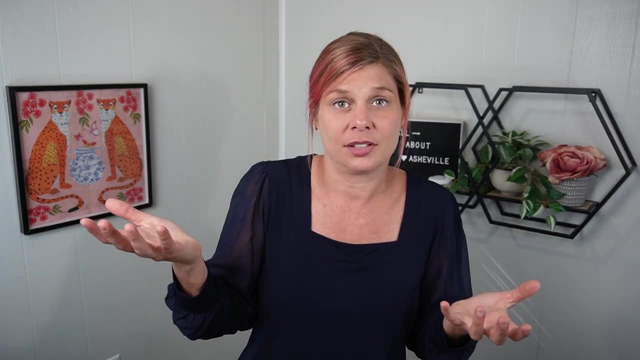 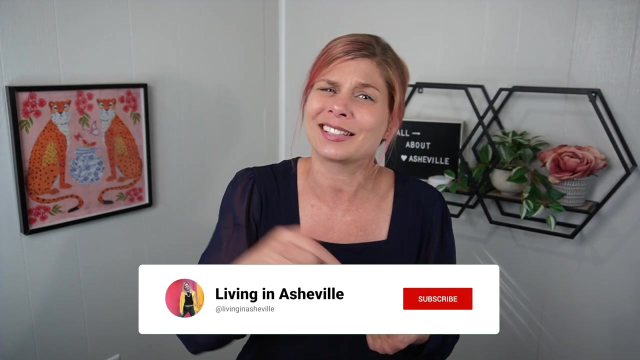 opportunities. both states offer their unique attractions and advantages, such as North Carolina's diverse landscapes and South Carolina's picturesque coastline, but ultimately, the choice of the two states depends on your priorities and your preferences. so if you enjoyed this video, don't forget to give it a thumbs up and subscribe to our channel for more insightful content. let us